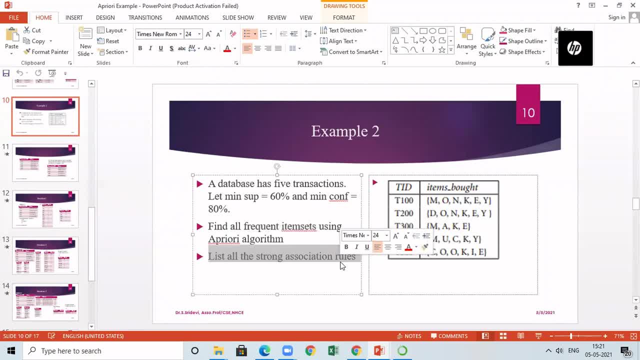 both the cases. So one function is used for finding the association tool in Python. We will see that, But for a priori one separate function. For FB growth, another function. So we are going to see this now. So first we are going to start with the a priori algorithm. 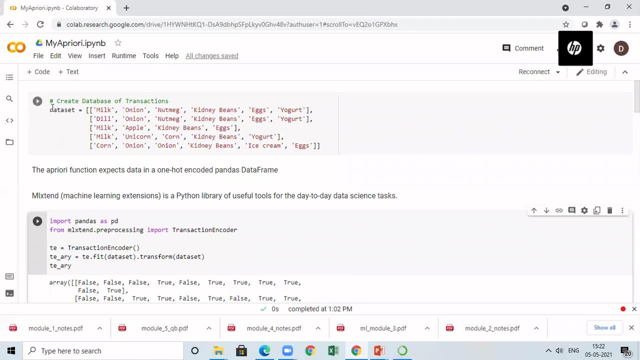 So this I am going to write and run in Google Colab. So in this first I am going to create a database of all the transactions. If you see, here we have seen that we have created a database of all the transactions. So in this first I am going to create a database. 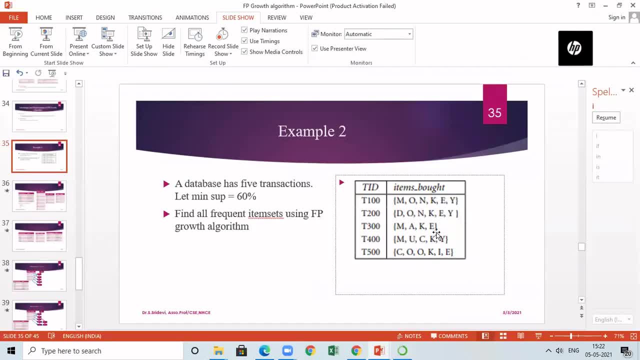 of all the transactions. If you see, here we have seen the example as this one Monkey donkey make monkey cookie and other things. So in actual database this is the first letter of all the items. This is the actual database. In monkey M stands for milk, O. 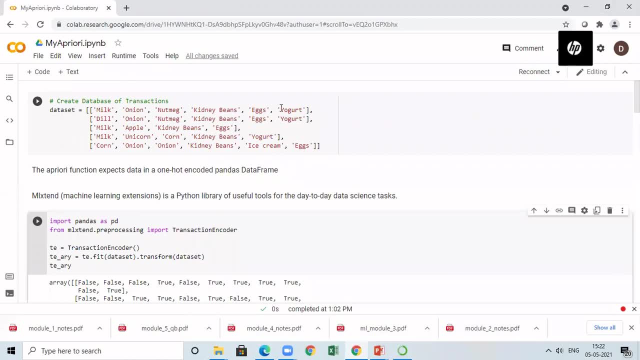 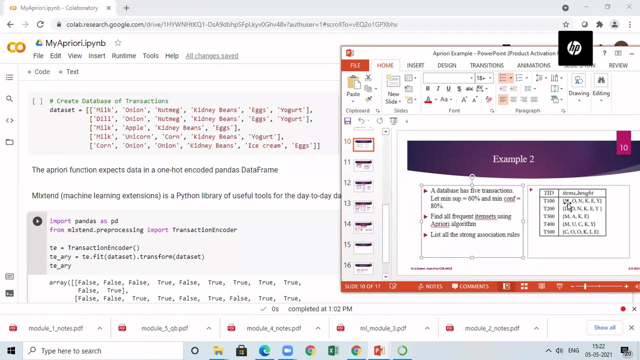 stands for onion N stands for nutmeg, and so on. So this is the data set. If you see how this is created, it is simply from this particular slide, nothing else. So I have a transaction here. If you consider T100, it is having totally six elements, All the. 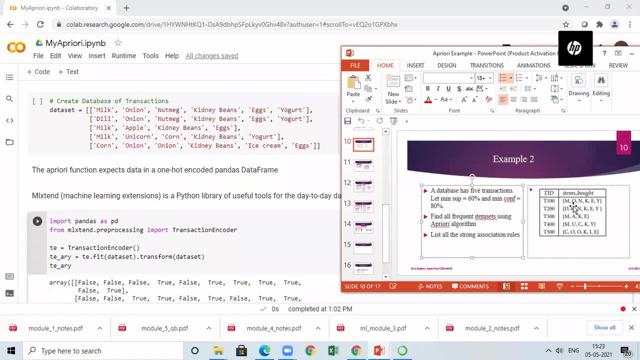 six elements are written as a list. Okay, we have a list of list, So I have a 2D list here. Then the second transaction contains donkey. that is six elements. So, if you consider this, we have six elements. This is for the second transaction. Then the third one is: 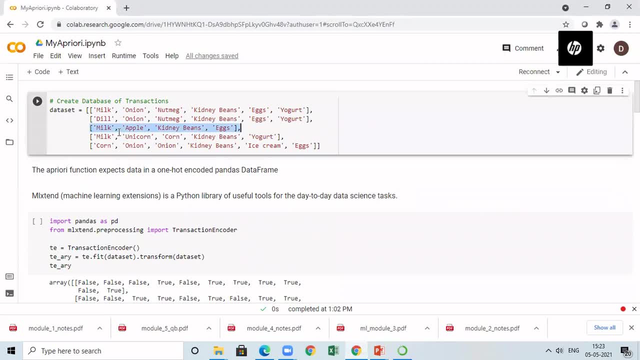 for the third transaction. It contains make M-A-K-E, milk, apple and so on. This is for the fourth transaction and then this is for the fifth transaction. So whatever transaction is given to you, you are going to create a data set containing all the transactions. 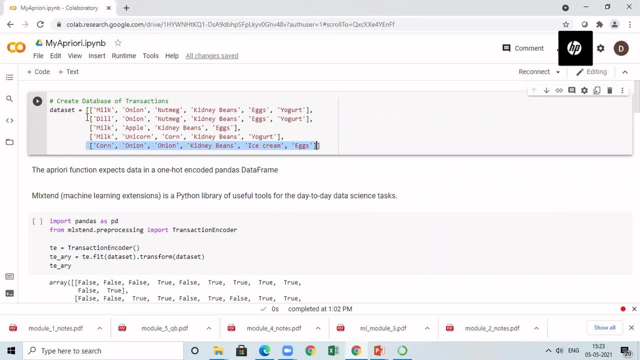 Here I have created a 2D list. Even you can create a CSV file and you can export that file and you can do the analysis. So now for simplicity, I have created a 2D list. Now I am going to use first Apriori algorithm. So in the Apriori algorithm when you want. 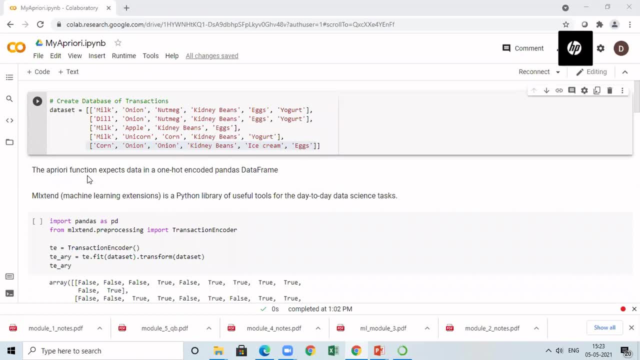 to start the built-in function for Apriori, you have to convert this information. Your data set should be converted into One-hot encoded Pandas data frame. Then only that particular function will work. So our aim is now: we are going to convert this data set into one-hot encoded Pandas data frame. 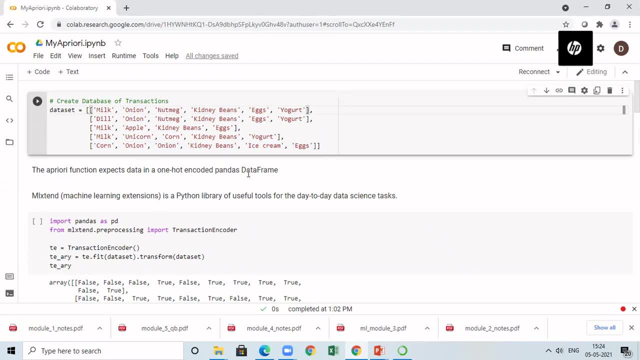 So for that we are going to import Pandas, Then we are going to import necessary libraries. So in this, to support the Apriori algorithm and then FB growth algorithm, we have a Python library which contains so many useful tools, and that library is ML Extender, So it is. 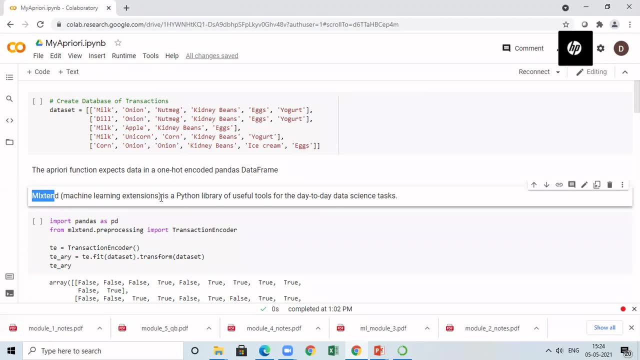 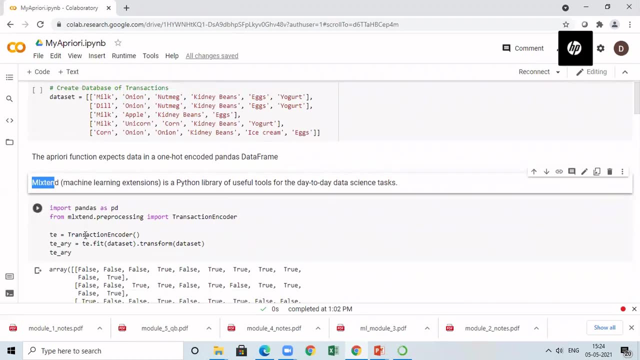 machine learning extensions. So we are going to make use of this Python library, which supports both Apriori as well as FB growth algorithm. So let us see the steps one by one. So first I am going to import Pandas as PD. After that I want to do now one-hot encoding. So for 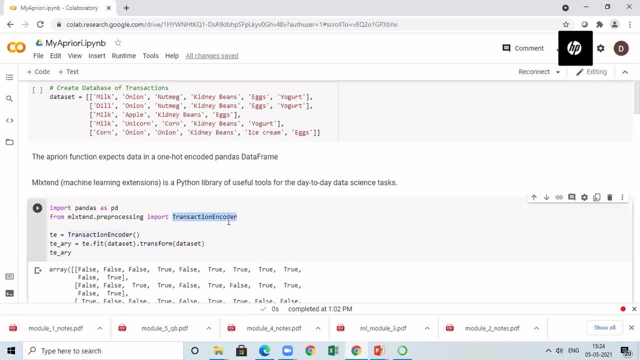 that I need to import transaction encoder. Okay, So this transaction encoder is available in this ML Extender, In that in pre-processing module it is available. So we are going to import. So I am going to write from ML Extender dot pre-processing import transaction. 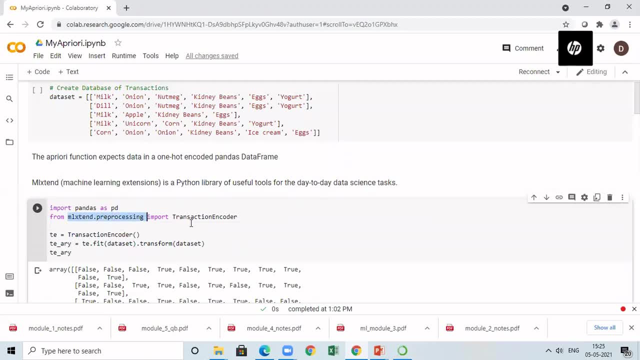 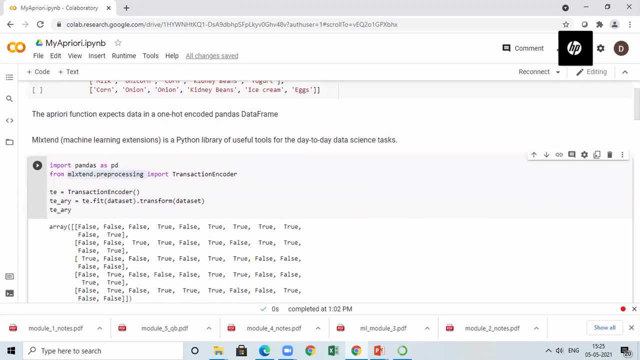 encoder. Actually this is a package From this. you can import this necessary things you want And once I import I am going to write my code for converting this into one-hot encoded Pandas data frame. So I need to convert my data set now. So for that I am going. 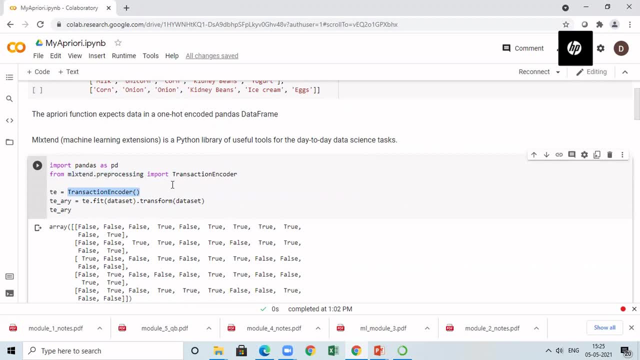 to create an object for transaction encoder, whichever I have imported here, and the object name is TE, Then I am going to pass my data set and with the help of this particular function I am going to convert that into one-hot encoding data frame. For that I need to call the fit. 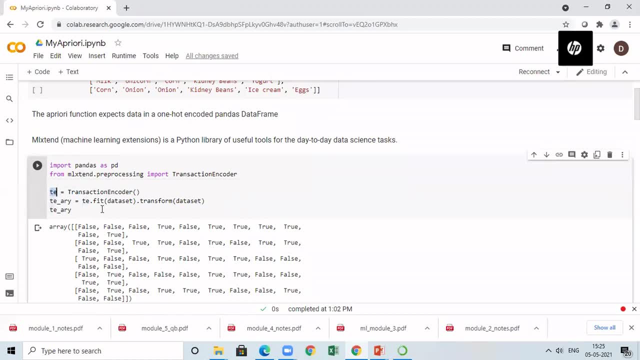 function. So with this object, TE, I am going to call the fit function. So you know, object oriented concept, With the help of the object only, I am going to call all the methods object name, dot, method name. So I am going to call now TE, dot fit. With this fit function, I. 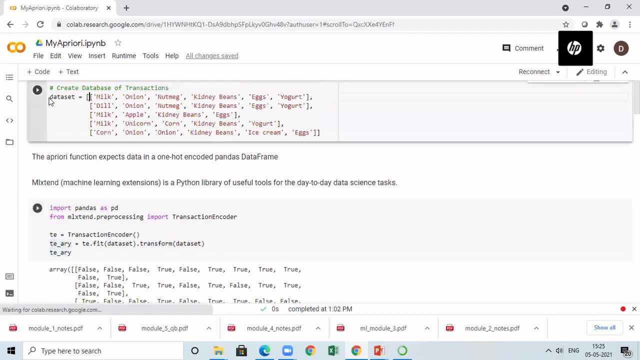 have to pass my data set. If you consider your data set, that is the data set. So you pass that object and once you do that, you need to transform it. So call now, transform again by passing the data set. Now it will convert your information. 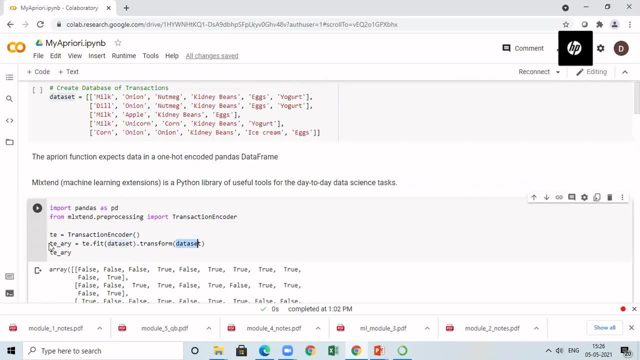 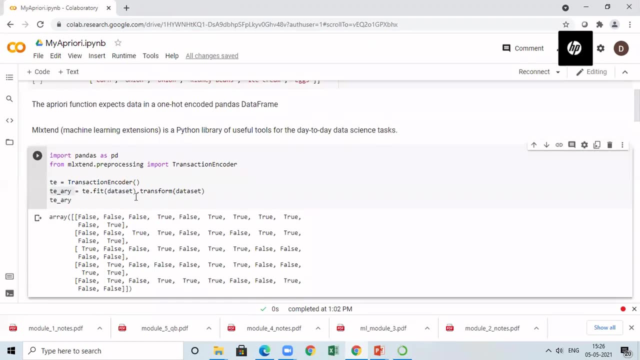 and your final answer will be available. You store that answer in another object. Here it is given as TE underscore ARY. Then I am printing this object so that you will understand what is the output here. You will understand what is one-hot encoding. So what is one-hot? 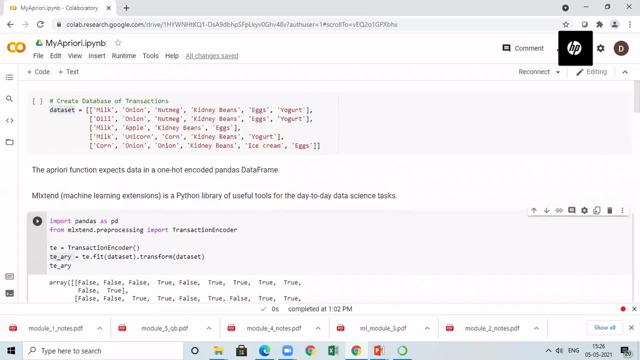 hot encoding here is: if you consider your transaction, it contains many items And when we started our apriori algorithm in the first table we have listed all the unique items. Unique item is nothing but milk is one unique item, then onion. second unique item: nutmeg. 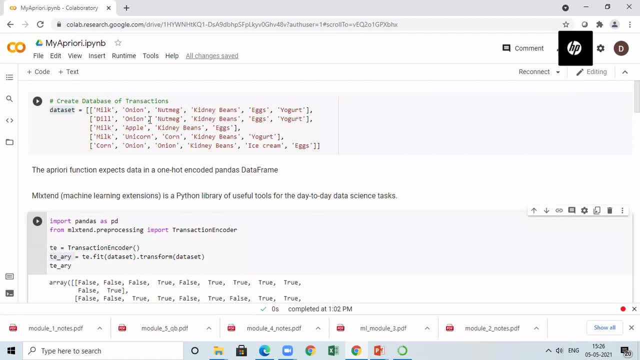 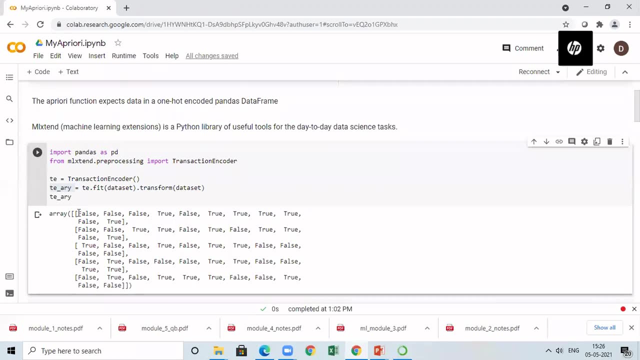 kidney beans and so on. There are so many unique items available. So in one hot encoding it will create so many number of columns Here. if you consider the number of columns in the first row, I have two, four, six, eight, nine columns. In the second here I have two. 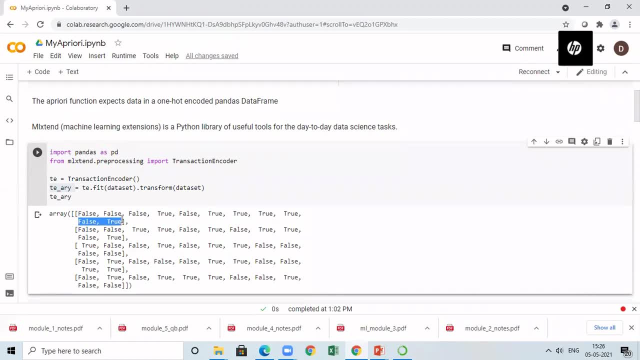 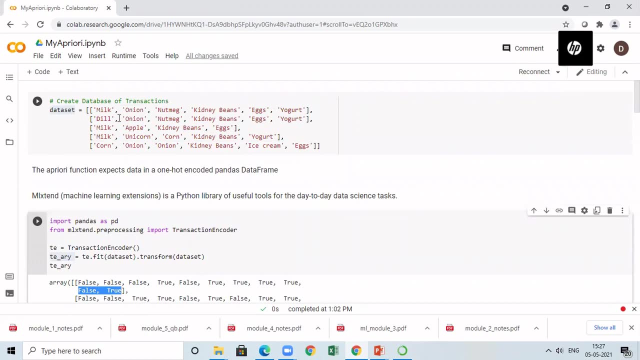 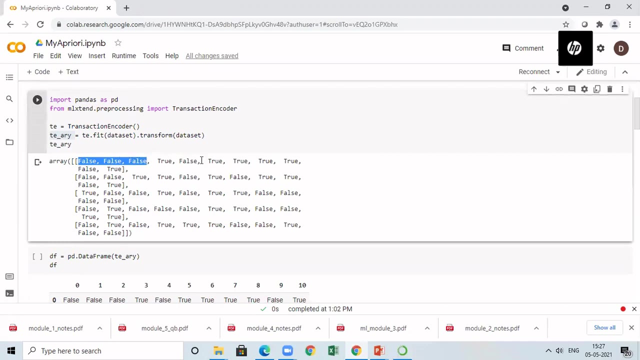 columns. So totally there are 11 columns. So what is the meaning of 11 columns? I have 11 unique entries or unique items in my transaction database. So you will have 11 columns And when you consider the first column you have something like false, false, then true and so on. So what? 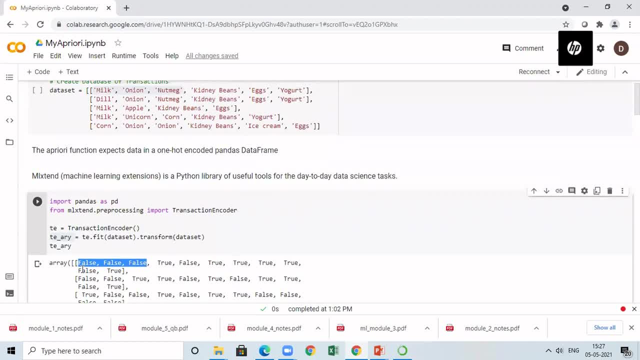 is the meaning of this. So if I have false for a particular entry, it means that that item is not present in the transaction. If it is true, it means the item is present in the transaction. So this is called as one hot encoding. So in one hot encoding it will create. 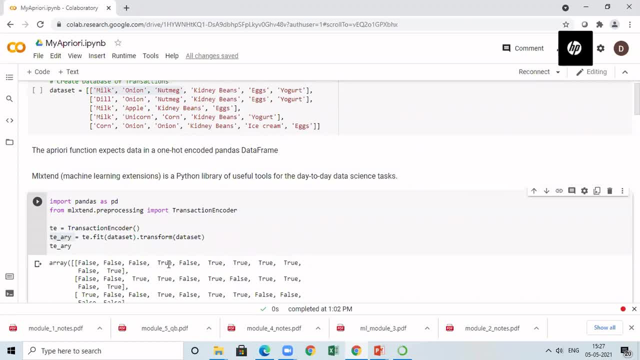 as many number of columns as that of the unique entries, Since we have 11 unique entries in the item set. we have 11 columns And, if you consider the first transaction, if a particular item is present, it will be written as true. If it is not present, it will be written as false. 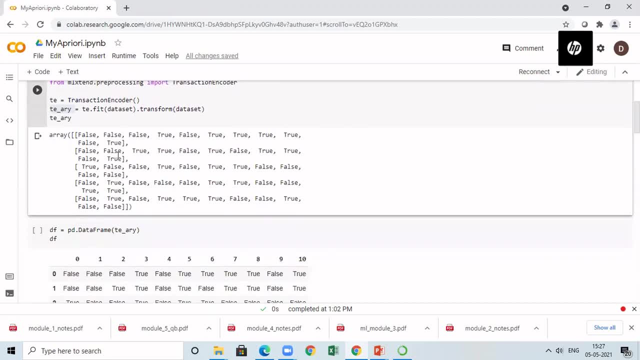 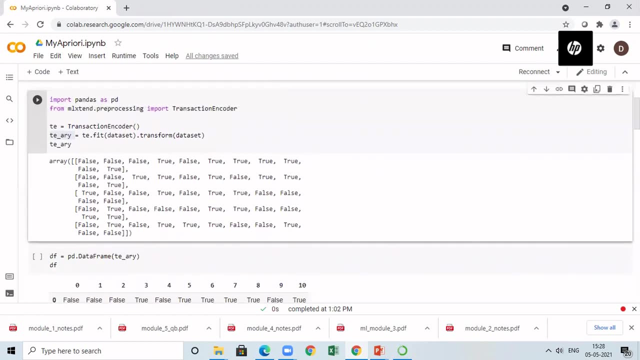 So now it is very difficult for us to understand the difference between false and true, So we are going to display the information in some other format. First let us convert this into Pandas data frame, because then only you can give that as into the a priori algorithm. So I'm going 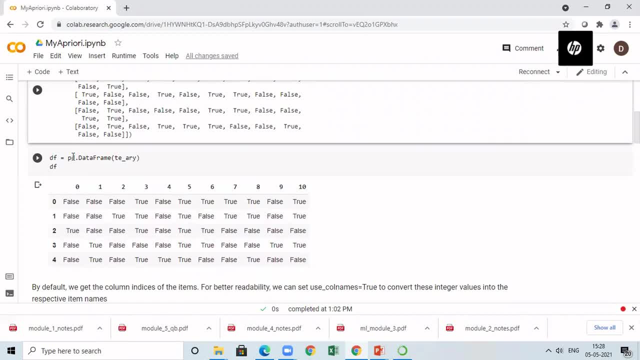 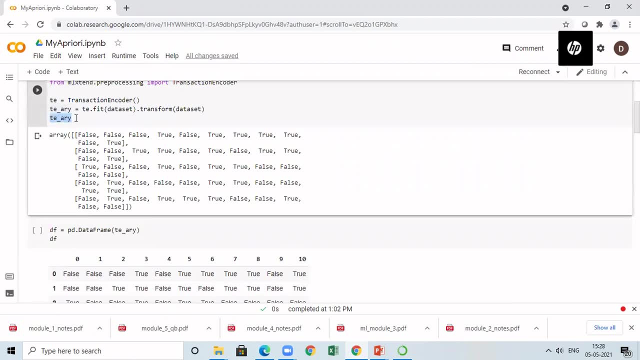 to convert this into Pandas data frame. For that I need to call pddataframe. I need to pass this one hot encoded information I have created That is nothing but te underscore array. I'm passing that. Then I'm creating a data frame, object df. When I list this data frame object df. 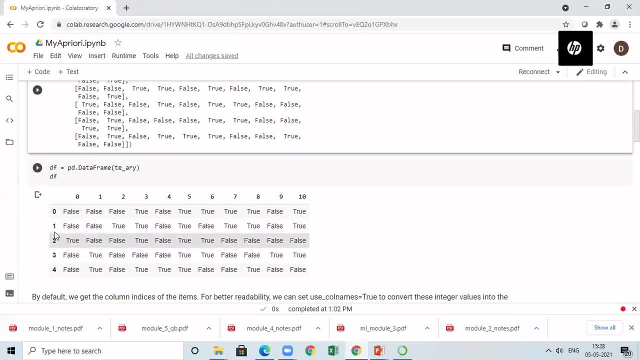 you will get some information like this: So what is the meaning of zero to four? It's nothing, but it will tell you how many transactions you have in your data set. If you consider your data set, or database, totally, we have five transactions. So I'm getting totally five rows here, one row. 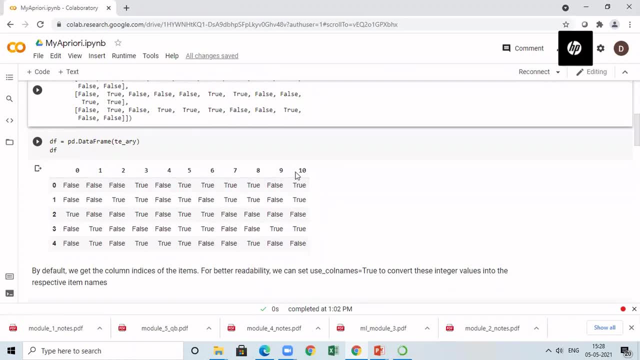 for one transaction. Then the columns is going to give you about a unique entry. So, totally, I told you there are 11 unique entries. So you'll have 11 columns, starting from zero index till the index 10.. So 11 columns are going to give you about a unique entry, So you'll have 11 columns starting. 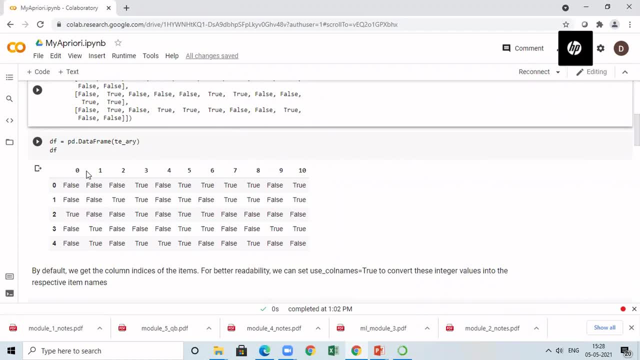 from zero index till the index 10.. So you'll have 11 columns starting from zero index till the index 10.. So you'll have 11 columns starting from zero index till the index 10.. Now still, we are confused. We don't know what is zero, what is one, and so on. Instead of displaying the index zero, 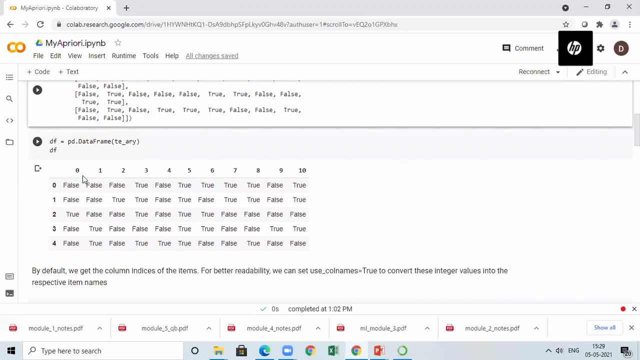 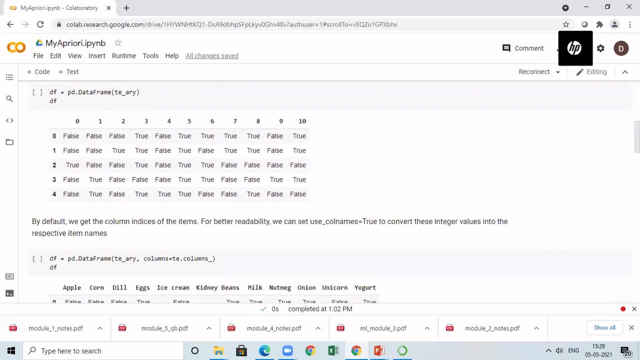 one, two, et cetera. if I display the actual column name, it will be easy for me to interpret the values. So for that, we are going to display the actual column name instead of the index. For that, the same function in this function when you convert that into data frame. 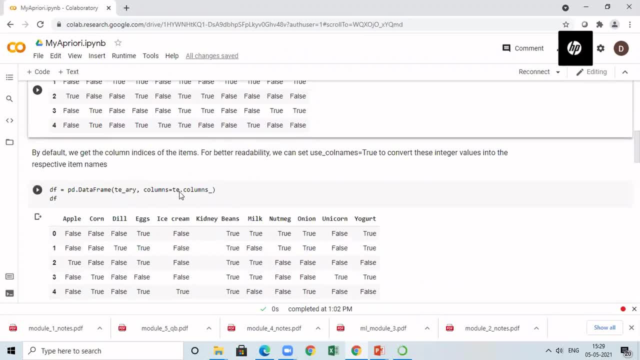 you can set something called as columns is equal to te underscore, columns underscore, So cecolumn is underscore. If you do that, if you set this particular attribute, then whatever is a column name, that will be displayed as such, so that we can easily interpret the data. Now, when you see, 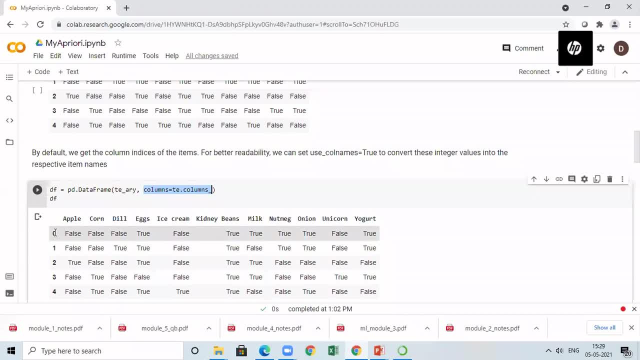 this one in the zeroth transaction. that is nothing but transaction number one, In that apple is not present. When there is a false in a particular column, it means that item is not present. Apple is not present, Corn is not present, Dill is not present, Eggs are present. 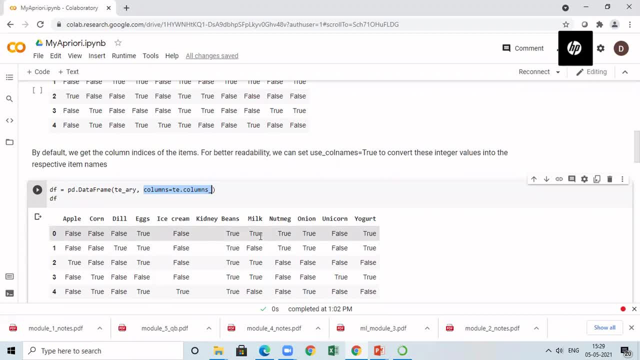 Ice cream not present, Kidney beans present. Milk present. Nutmeg present. Onion present. Unicorn absent And true Yogurt present. Whenever there is true, it means that item is present. Okay, If you check wherever you have true, you will get the letters: monkey M-O-N-K-E-Y. 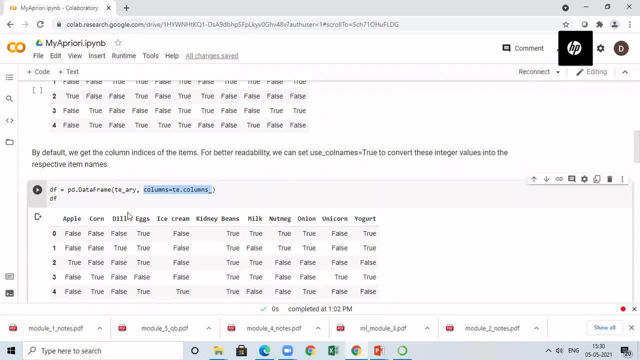 Okay, Similarly, for all the transaction it is printed. This is called as one hot encoding. So in one hot encoding you will be creating number of columns which is equal to number of unique items, And if a particular item is present, we are going to write that as true If an item is. 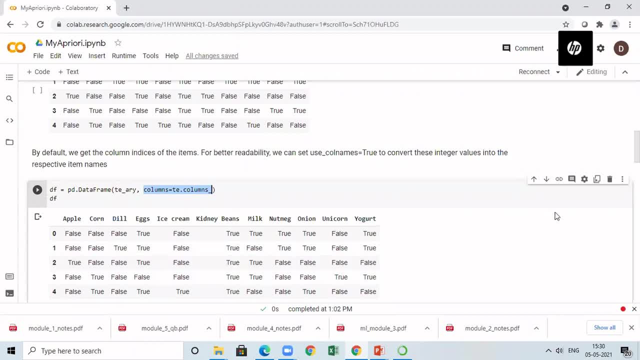 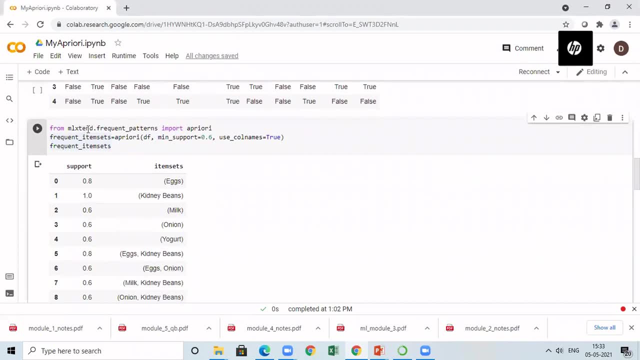 absent in that transaction, we are going to write it as false. So now we are going to see the a priori algorithm. So our a priori algorithm is defined in MLxtent, So we are going to import it. So from MLxtentfrequent underscore patterns I am going to import a priori. After that: 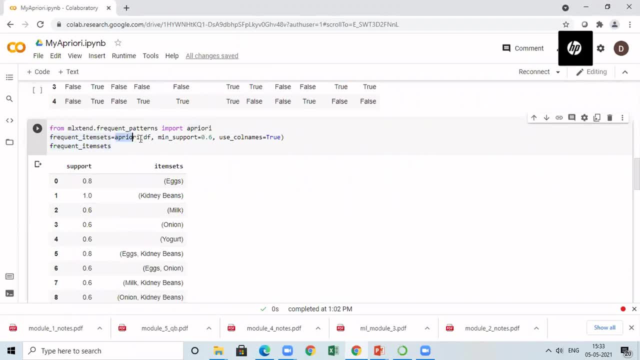 I am going to call the algorithm. that is the function a priori. For this function, we are going to pass the necessary arguments. The first argument you have to pass for this function is: where is your data set available? Now, my data set is available in the one hot encoded format in the data frame DF. 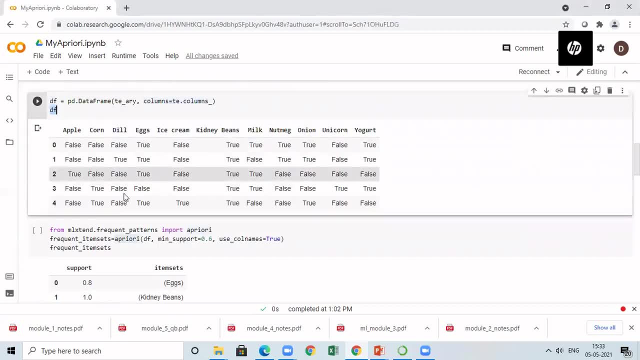 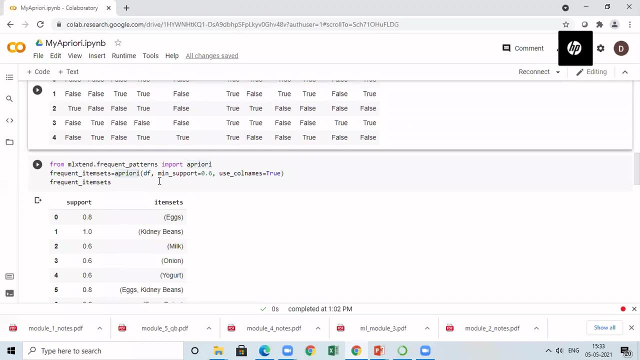 This only. we have created in this step DF So that you have to pass as the argument. So I am passing DF as one of the argument And this a priori algorithm. next accept another argument. that is nothing but minimum support. So you have to give the minimum support now. 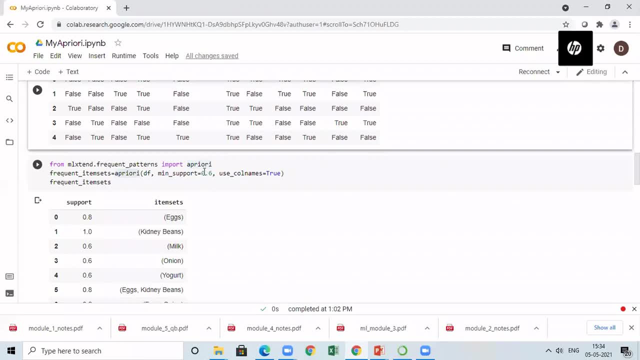 According to our example, our minimum support is 60%, So I am giving now 0.6.. After that, use underscore call names. I am setting this as true. Let me remove this so that you will understand why I am going to set this. Now. let me run. 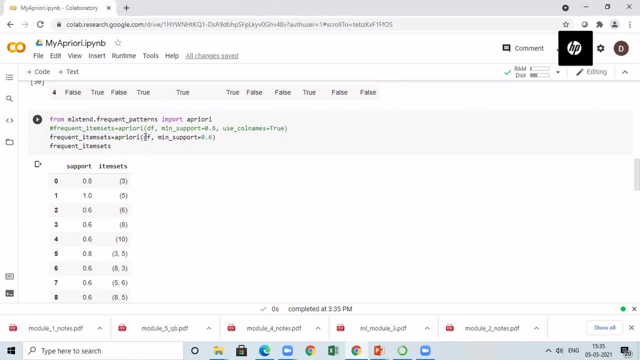 Here. if you see, I am running this by passing only the data frame and then minimum support is 0.6.. It will return me all the frequent item sets, whatever we have generated in the example. that will be returned to you. You just display them by calling frequent underscore. 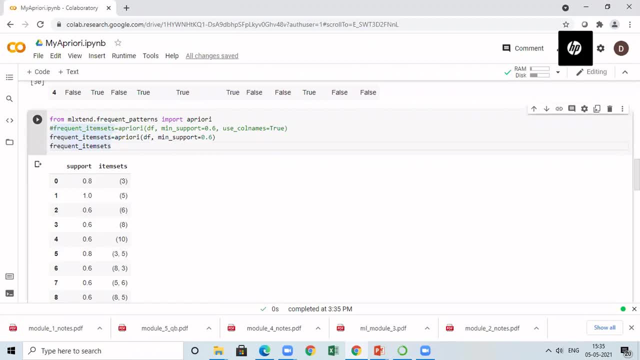 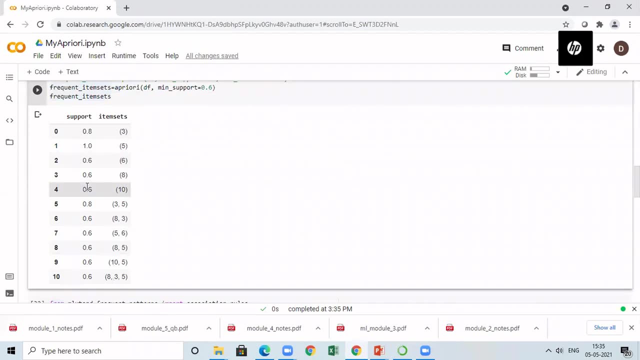 And I am displaying this. So it is showing me something. I can't understand anything from this. It is actually displaying the frequent item set. whatever we have derived in the algorithm, that is displayed, But we are not able to understand anything because it is displaying. 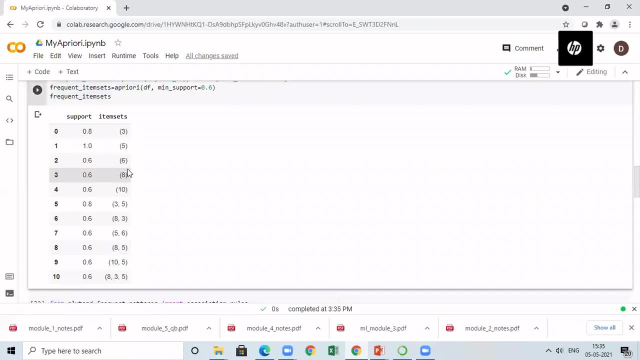 me the index as three, five, six and so on. I don't know what is the exact item, So I want the item instead of the index, for that only I have given this. So now let me comment this, Let me do this one. 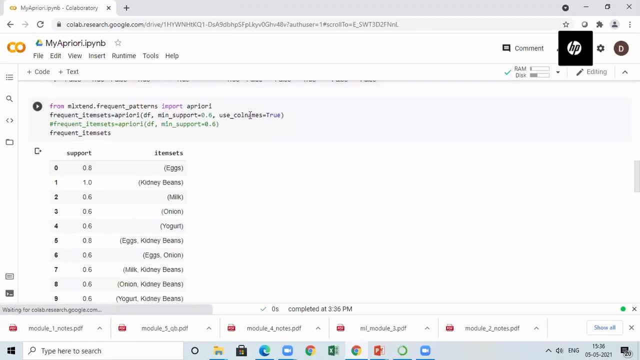 So When I do this now here, what I have given is use underscore call names and set as one. It means that whatever is a column name for your data set like here. if you consider the column names are Apple, Corn, Dill, et cetera. 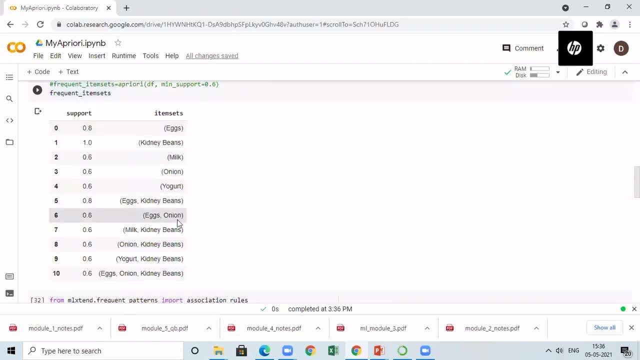 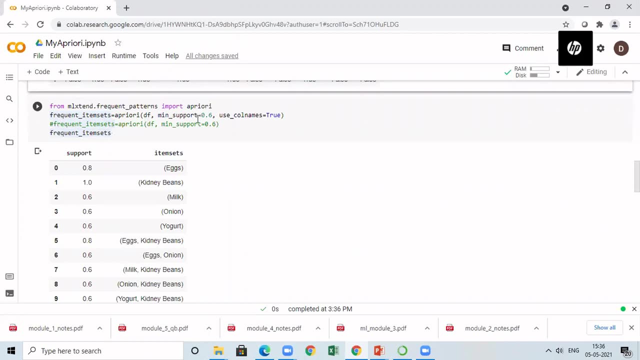 So all these column names will be displayed instead of the index. So that is easy for us to understand. So we are going to set this. So I am calling a priori by passing three arguments. One is a data frame. Second is a minimum support. 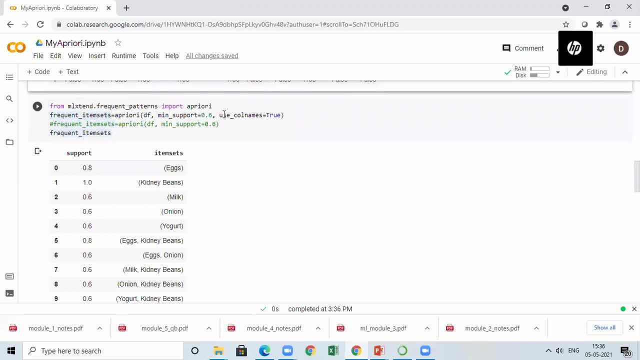 Third one is I am going to display the column names instead of the index, That I am setting this as true, It will be converting and the algorithm will run. Then, finally, you will get the answer, which is nothing but frequent item sets in your 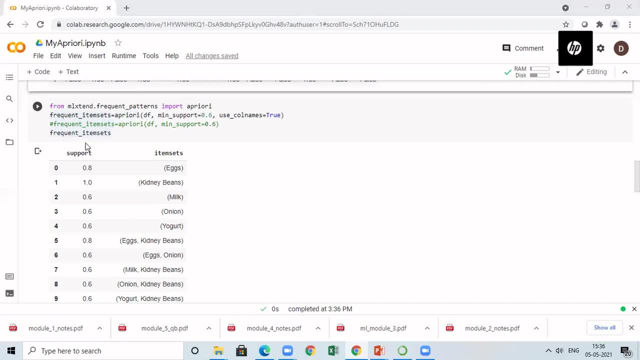 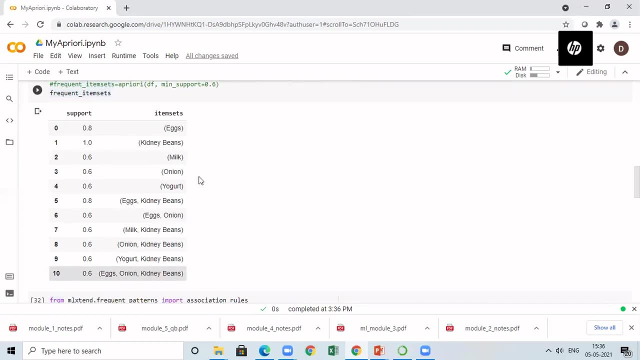 database according to the minimum support: 60%. So you display that If I display frequent underscore item set, I am getting these things. So what is this? How many items I am getting? When you remember, in the previous example we have seen that when we run the example. 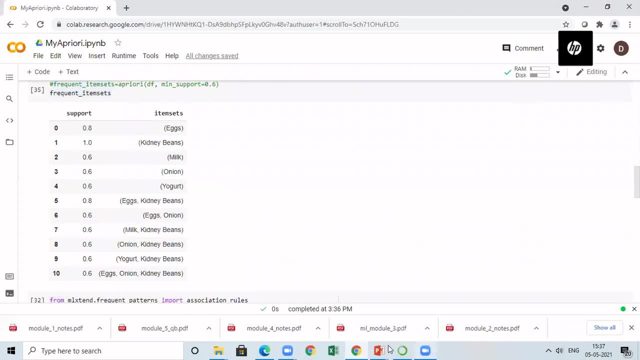 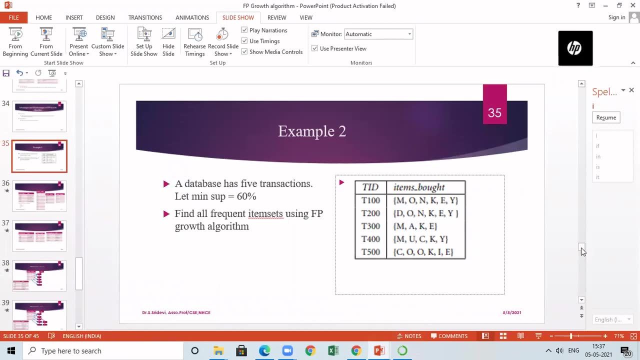 we got totally 11 frequent item sets. Let me show that so that you will understand. So for both algorithms the output is same. I will take the FP growth algorithm. So here we constructed the frequent item set. at the end, Totally 11 items are there in the frequent item set. 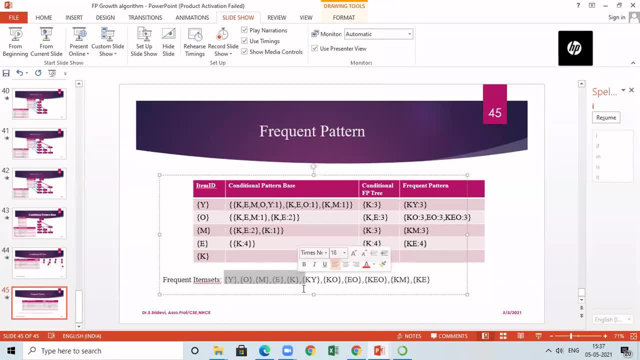 So if you consider, in one item we have five items totally, Then in two items we have five items total, Then in three items we have one. You remember the three items so that you can take it: K E O. 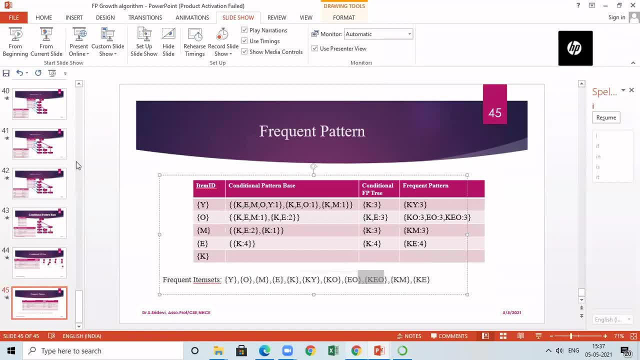 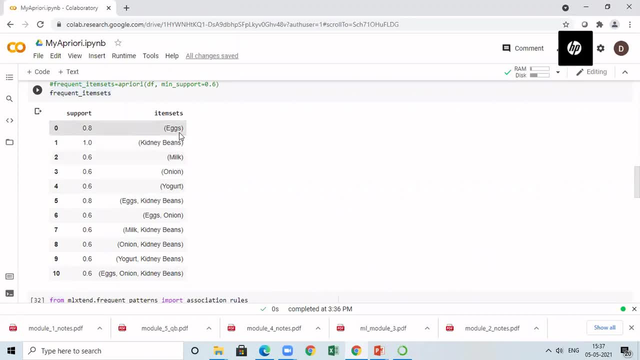 Key letters are present. Now let us check the output here. Totally, 11 items are present, 0 to 10.. And in that, if you consider one item set, we have five. one item sets X: kidney beans, milk, onion yogurt. 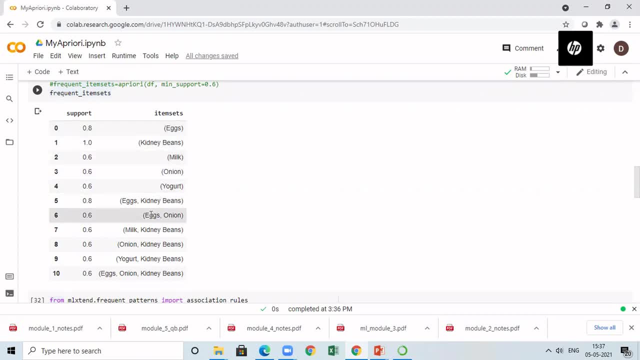 That is nothing but E K, M O Y. Then, if you consider two item sets, we have X kidney beans. That is nothing but E K. Then we have E O, Then we have M K, O, M O K and then Y K. 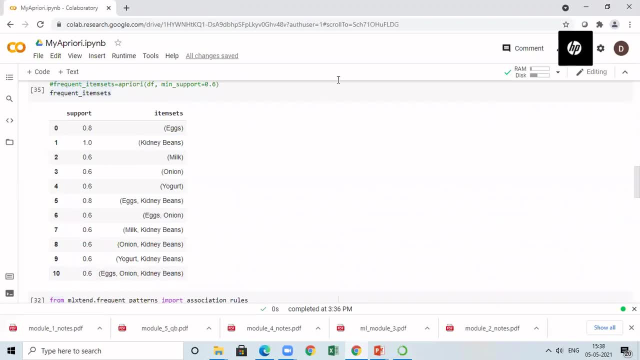 And if you consider three item sets, we have egg, onion and then kidney beans, So totally we have displayed 11 items. So this is nothing but the output of the a priori algorithm which is generating 11 frequent item sets. 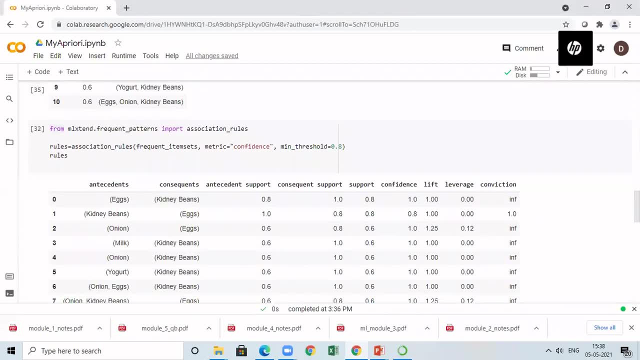 So now the first part of the algorithm is over. Our second part is we have to generate the association rules. So association rules are nothing but the rules of the form. A implies B. It means that when I buy item A, what is the probability that I will? 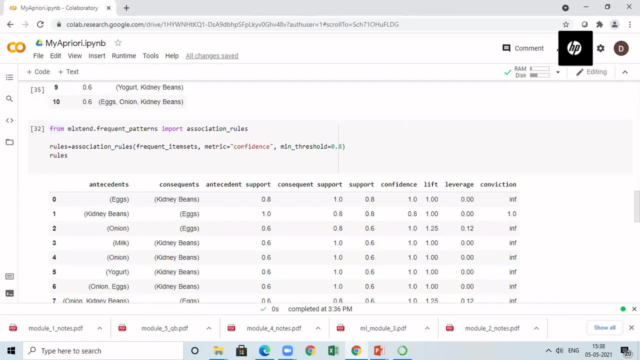 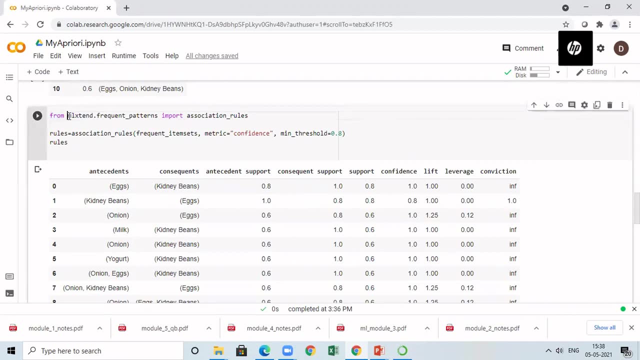 also buy item B in my transaction. So you have to generate the association rules. and for generating association rules again in the ML package, ML extend- you have frequent underscore patterns In that we have a module called association underscore rules you can import. 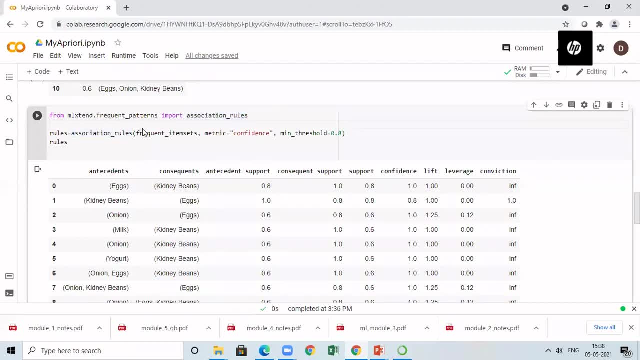 So I am writing now from ML extend dot. frequent underscore patterns- import- association underscore rules. When I do that, all the necessary packages will be imported. Now I'm going to derive my rules. So for deriving my rules I have to pass my frequent item set. 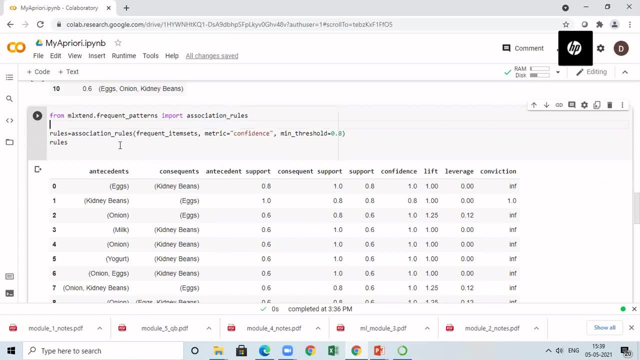 If you consider first, we have generated the frequent item set that should be given as input to the association rule algorithm. So if you consider the input, it is not data from DF, instead whatever you have generated in the previous step. here we have the output of the a priori 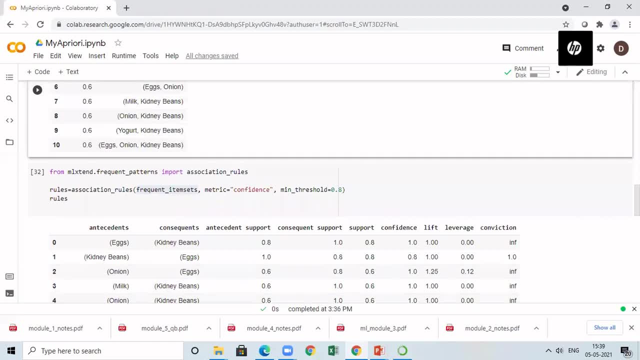 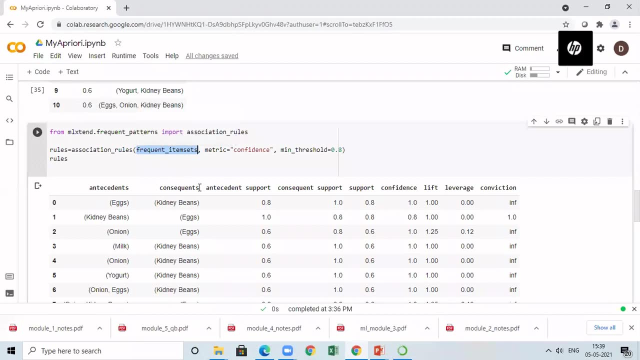 algorithm is stored in frequent underscore item set that should be given as input. So I'm giving that as the input. So accordingly it will generate all the association rules And remember, for the association rules you have to set the confidence. So for the confidence there is a minimum. 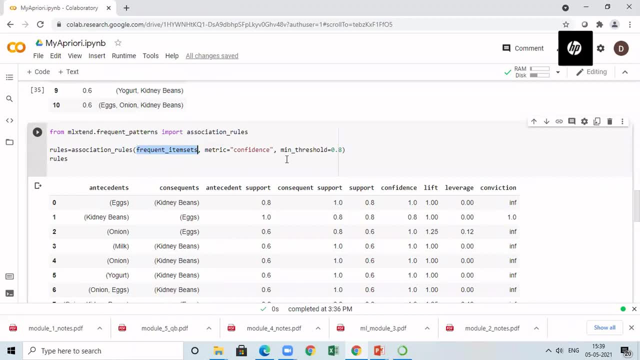 In our example it is given as 80%. So I am going to now set the minimum threshold for the confidence as 80%. So I have to give the metrics as confidence, because this minimum threshold is for the confidence. So set now metric is equal to confidence and then set the minimum threshold for this as 80%. 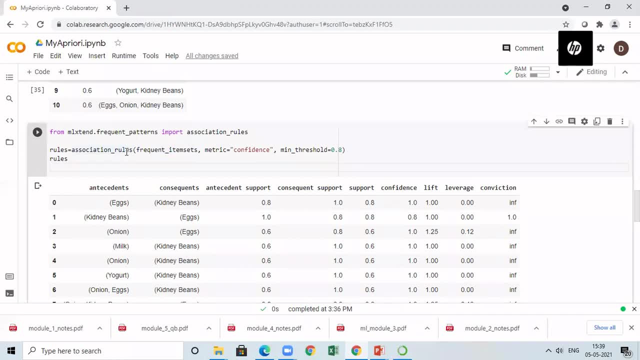 That is 0.8.. And once you do that, you can call this algorithm, You can call this function. It will generate all the association rules And it will return that rule to you. You store it in a data frame. So this rules is a data frame which will store all the answer. 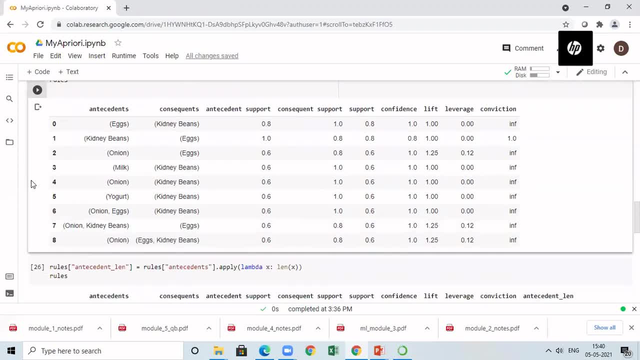 You can display the data frame now And when you run. you will get all these things. If you see, all are not important to us. we will focus on certain things. You consider this. There are totally 0 to 8. That is totally 9. association rules are there. 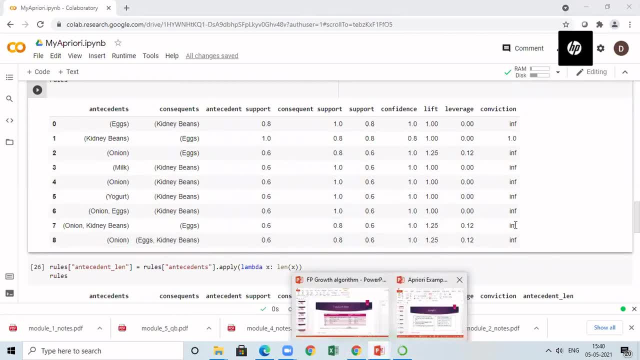 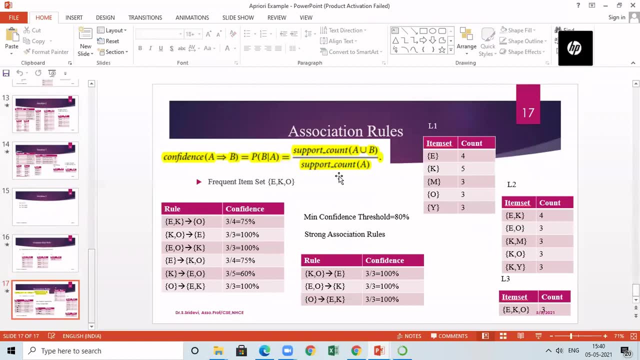 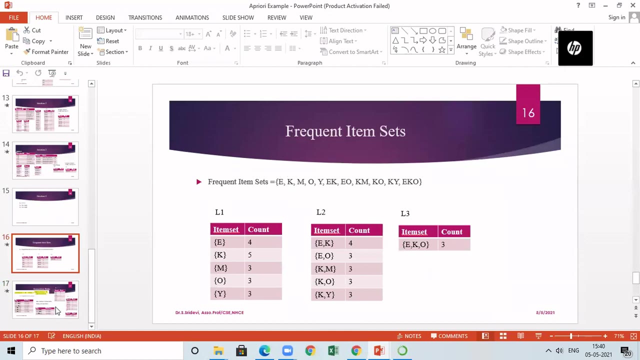 But if you consider a priori example, what we have seen in the class, I'll show you that First, then we will come here so that you will understand. So when we check the association rule, actually we started with the frequent item set. that has given us input to the association rule. 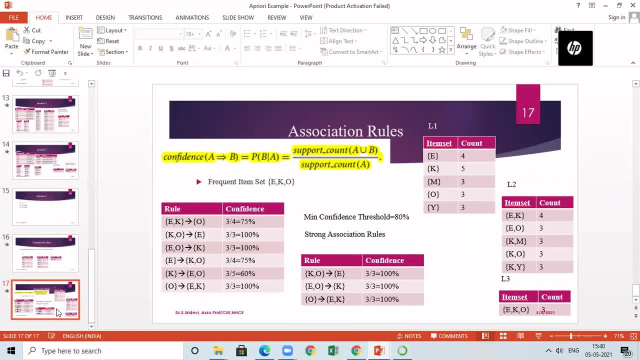 Then we set the minimum confidence threshold. Finally, we came up with the rules, And in this algorithm we have seen that only three rules are there. First rule is K- O implies E, Then E- O implies K, Then O implies E- K. 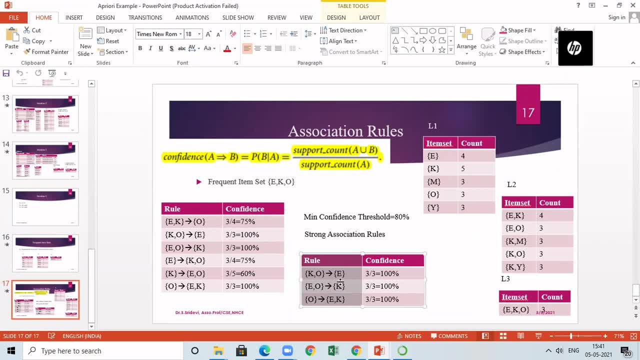 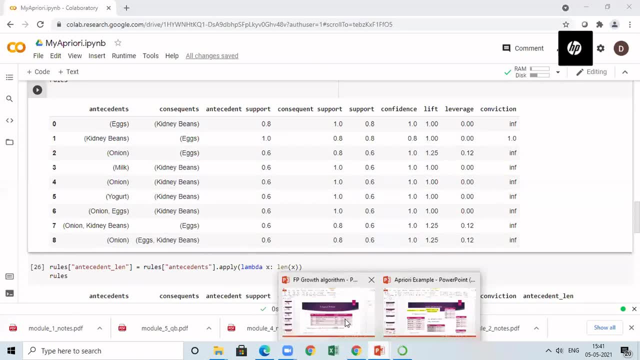 Then E O implies K, Then O implies E, K. Only three rules are there, But this should be displayed to you Now if you see your output totally. we have nine rules. Where are these three rules? Let me keep it here so that you can see the output. 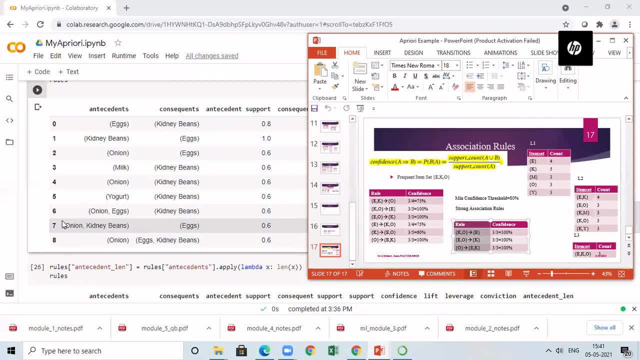 If you see this focus on the last three rows in this. The first rule here is: onion X implies kidney beans. So that is here. The second one, onion X implies K. And if you consider the seventh one, onion Kidney bees: kidney beans implies X. 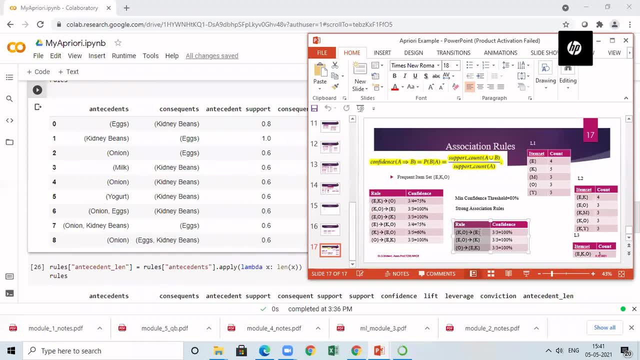 So that is the onion. Kidney beans implies X, the first row, And if you consider the last one onion implies X- kidney beans, That is here. O implies E, K. Okay, So these are all the rules we have derived in our algorithm. 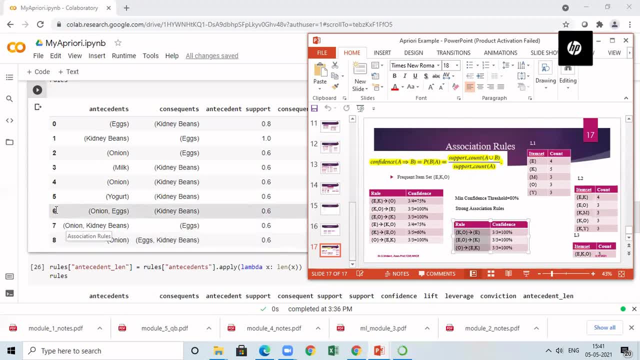 But here, in addition to those three rules, it is displaying them correctly- In addition to those three rules, it is also displaying some other information. So what does this information is? Uh, we didn't, We didn't consider the one-to-one mapping. 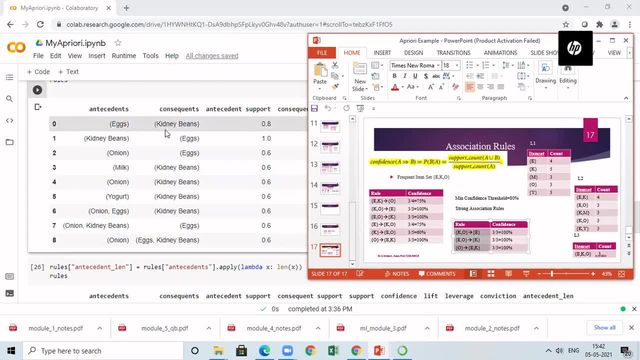 So whichever one-to-one mapping is satisfying this information, that is also displayed When we consider this. I told that if you have totally three items, uh, if you write two items in the left-hand side, the remaining one item will appear in the right-hand side. 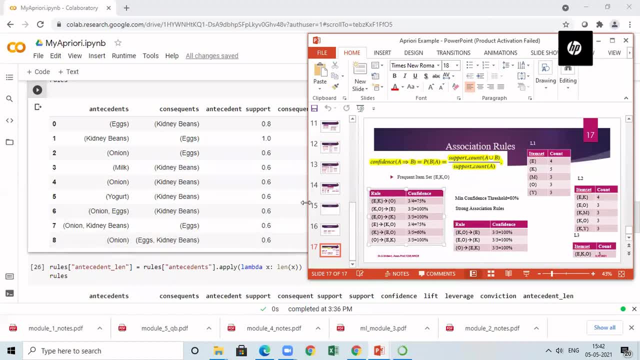 So we proceeded like that. Here it is displaying that, in addition, if you have one-to-one mapping, that is one item here, one item in the right-hand side, So the third item will not be present. So that is also listed in addition. 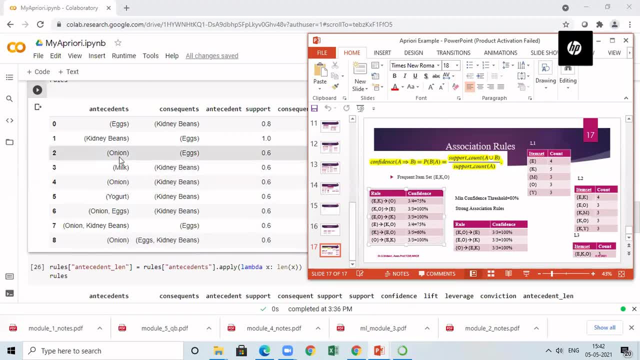 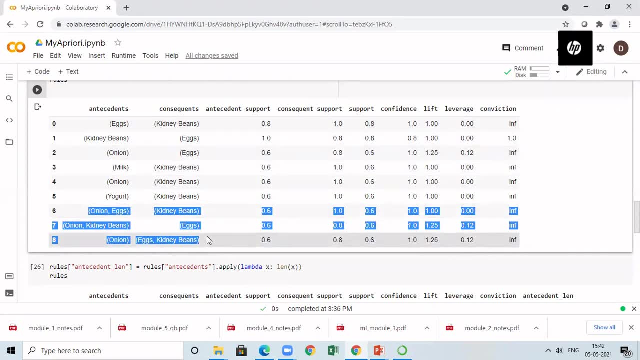 In addition to our actual strong rules. Okay, It is not wrong, It is correct, It is. This is the actual output we want in our algorithm. In addition, it is displaying this type of relation also. Okay, So in the algorithm, uh, in the three rules, we have the confidence as a hundred percent. 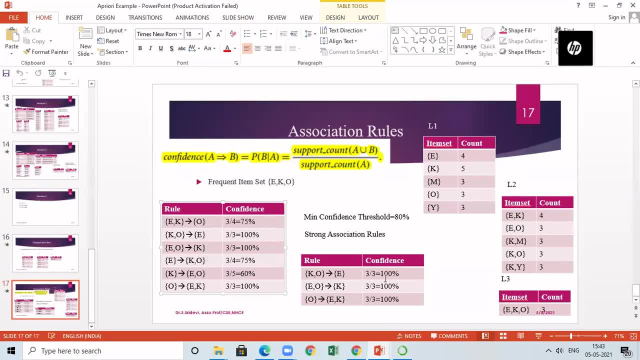 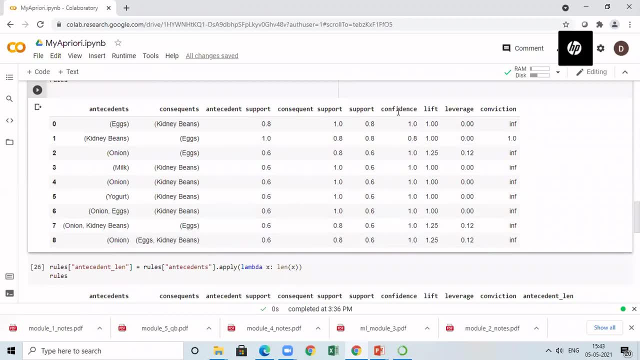 We have derived that in our algorithm. Now let us check whether we are getting the same confidence when we run the program. Also, if you consider, the last three rows correspond to the item in our program. if you consider this column- confidence- there are so many columns. 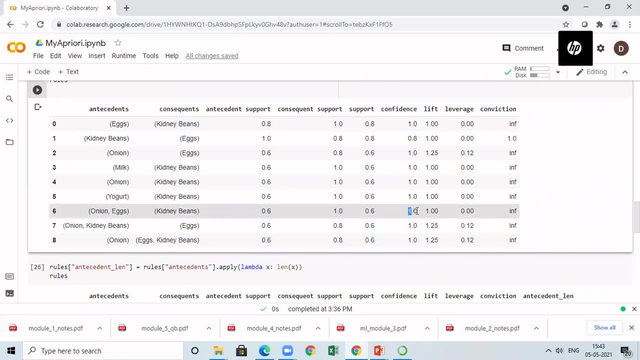 Okay, Don't worry about that. You consider the column confidence. If you see the confidence here, it is 1.0.. That means that a hundred percentage confidence. So this is the association rule you can generate with the help of this function. 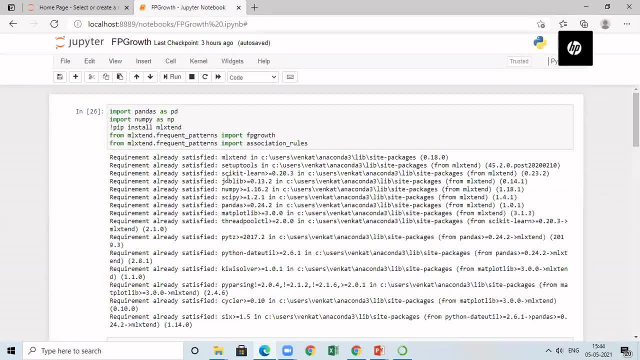 You consider the FP growth algorithm. This algorithm I'm running in Anaconda. I'm importing now again the ML extend package only in that only this algorithm is also present. So, uh, when you run, if you don't have any package, you know how to install it by means of pip install. 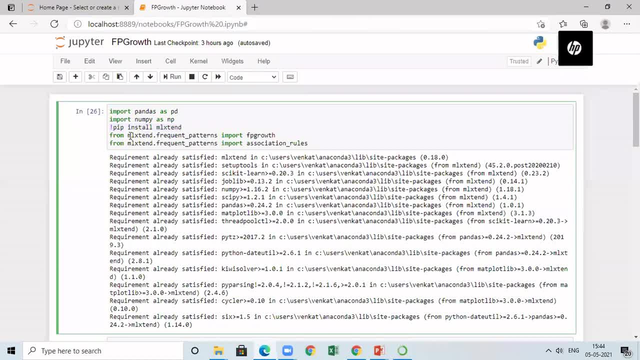 You can install any package, whatever You want. So here I want ML extent, So I'm installing that in that I have frequent underscore patterns in that only this FP growth is also there, So I'm importing that. then association tools I want later in my algorithm. 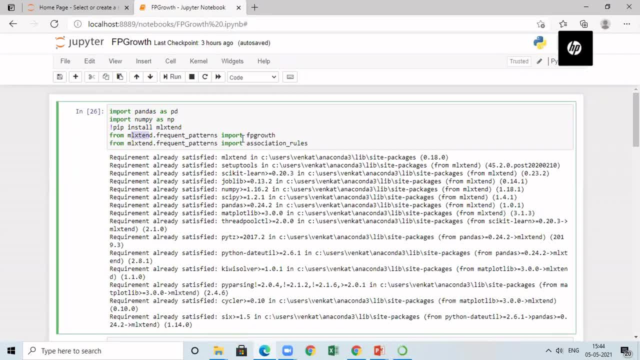 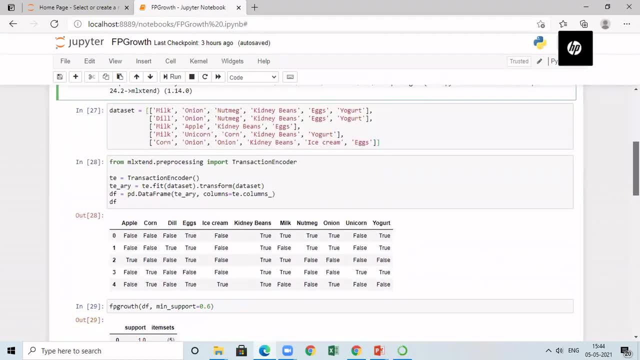 So I'm importing that also. So I mean I have imported two things now: FP growth and then association tools. both are available in ML extent. Now I'm considering the same data set Now first I'm converting that into one hot encoded file. 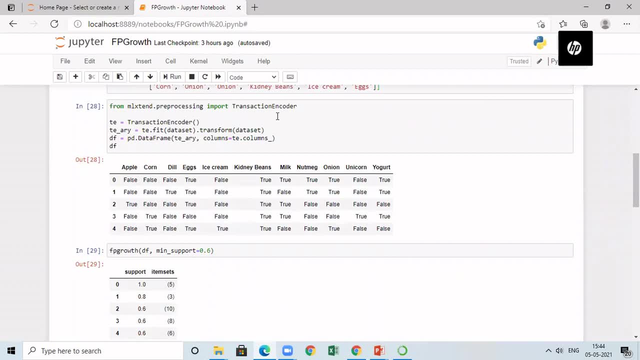 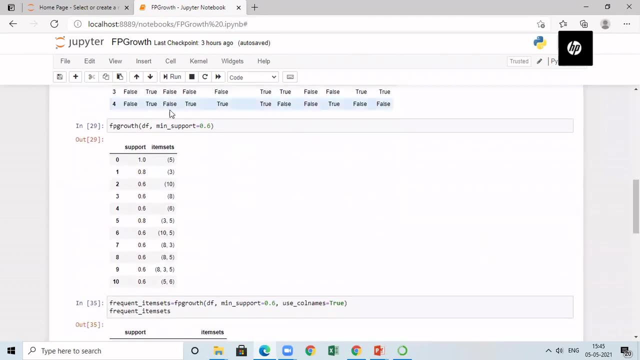 Format, because even the FP growth algorithm need your information in one hot encoded data frame. So we are converting that up to this It is similar, So one day this part is different. Now we are going to call the FP growth algorithm. 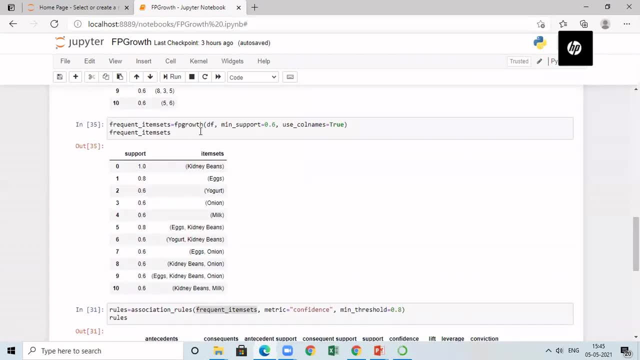 So now I'll show here. So I'm going to call the FP growth algorithm. So in this again we have to pass three arguments. The first argument is the data frame which contains your data. Second, specify the minimum support. Third, if you want to see the column names instead of the index specific, use underscore call names as. 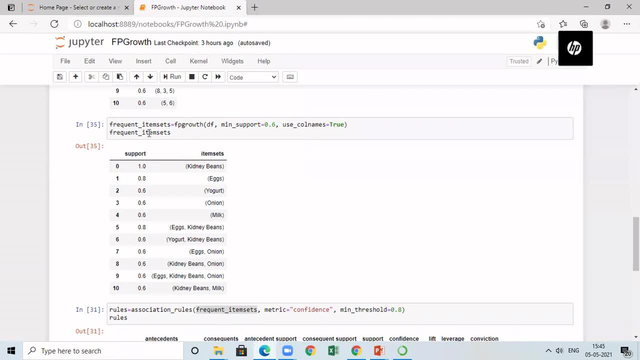 Now it will return you a data frame, store it and then displaying it. I'm getting the output. If you consider it is same as a priori algorithm. So totally, 11 entries are there. 11 frequent item sets are there. 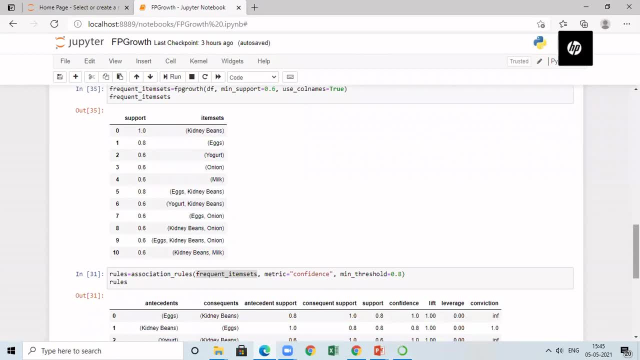 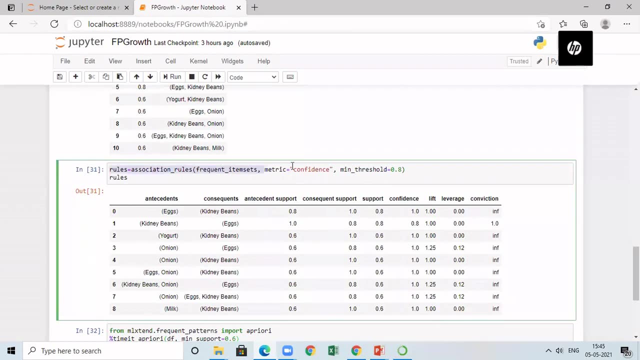 OK, so the output of FP growth algorithm is same as a priori, And then association tools: same thing. Whatever I have done in the last example, the same thing I'm doing here. I'm setting the metric as confidence And I'm going to set the minimum threshold only for this confidence. 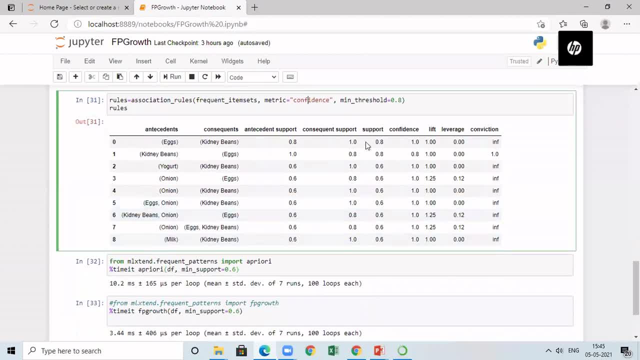 It is set as 80%, Again we are getting the similar ones. Now comes the important thing. When I teach you the FP growth algorithm, I told you that in case of a priori algorithm, we are going to do so many scans in the database that is going to increase our time. 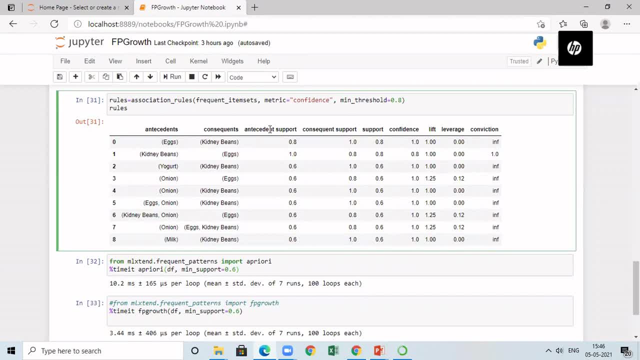 So our aim is: we want to reduce the number of scans. For that only, we went for the FP growth algorithm. Now you can check the running time of these two algorithms And you can find that FP growth algorithm will run very fast when compared to a priori algorithm. 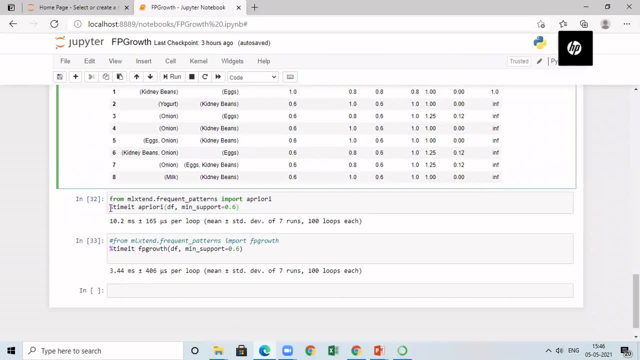 So for that I'm going to use a magic function in Python. You might have studied this one Time it. This is a magic function with the help of which you can find out what is the execution time of a particular step or otherwise, a particular function or a program. 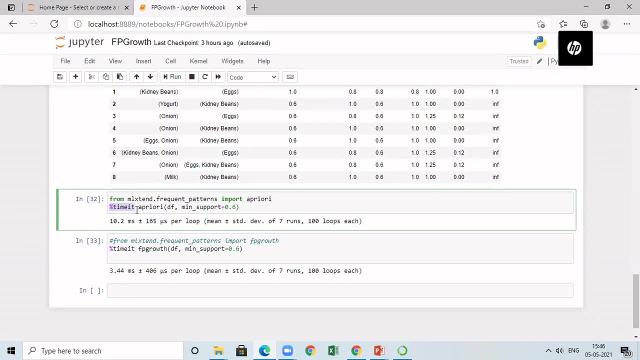 So that is possible with the help of this function, So I'm going to use that now. So first I'm going to find out how much time is taken by a priori algorithm for running for this particular data set. So I'm going to call a priori. 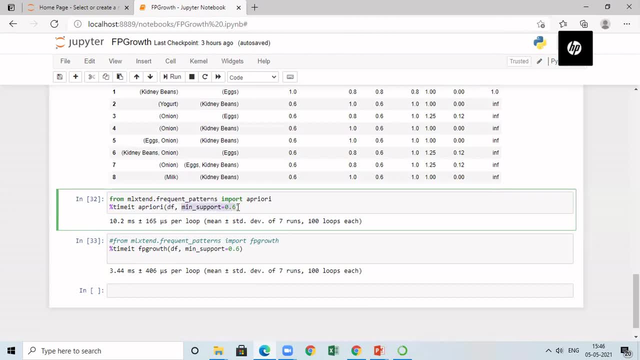 I need to pass. If the data frame, then I'm setting the minimum support as 0.6.. It will call the algorithm. My algorithm will run. I want to find out how much time this algorithm will take to run on a particular data set which is nothing but df. 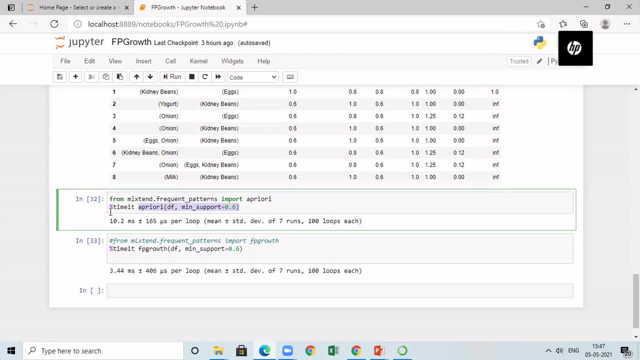 So for that I'm calling the magic function. So for that I'm specifying first at each time When I run this step. I'm getting this as an execution time: 10.2 milliseconds. Now I want to find out what is the time taken by FP growth algorithm for the same step. 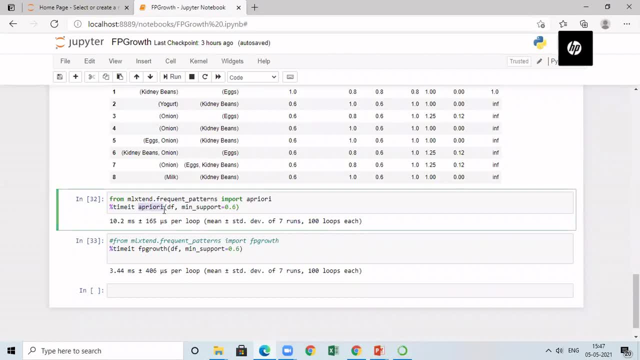 So now, instead of a priori, I am calling FP growth algorithm with the same input df min underscore support as 0.6.. I want to find the running time again, So I'm calling first at each time. 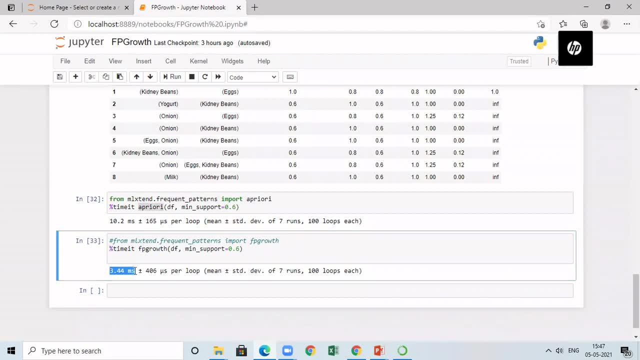 Now, if you consider this time, it is now 3.44 milliseconds. So, if you consider both, both are working on the same input, But my a priori algorithm is taking 10.2 milliseconds, whereas FP growth algorithm is taking 3.44 milliseconds.